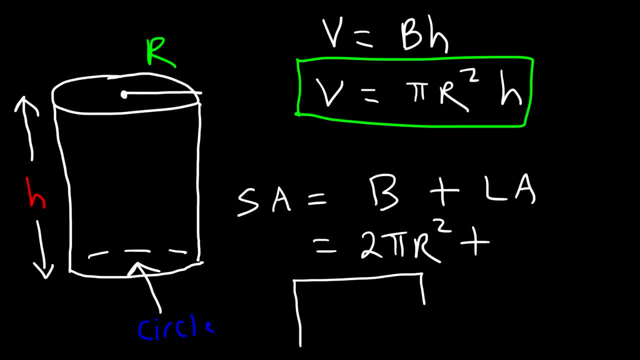 Now, if you take, let's say, a piece of paper, you can roll it into a cylinder. Let's say, this is still the paper, but it's about to be rolled into a cylinder, So the rectangular area of this paper can form the size of a cylinder. 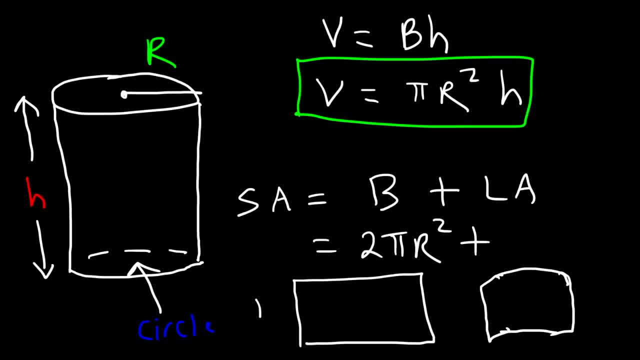 That is the lateral area And we know this is H, And the length. if you turn it into, if you roll it up into a cylinder, that length highlighted in green becomes the circumference of the cylinder. So basically it's the perimeter around the circle. 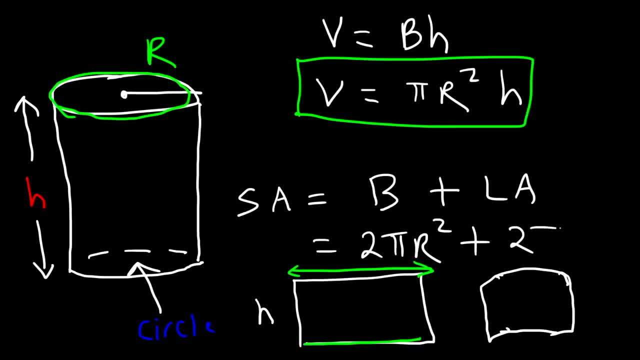 So therefore it's going to be the circumference, 2 pi r, Which represents the length in green times the height. So that is the surface area. It's basically the area of the base, That is, the area of the circle on top and the bottom, plus the lateral area. 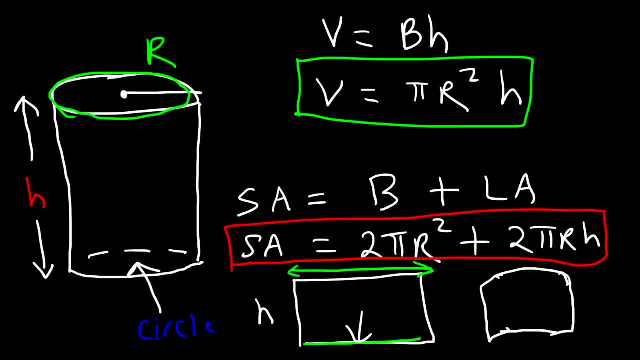 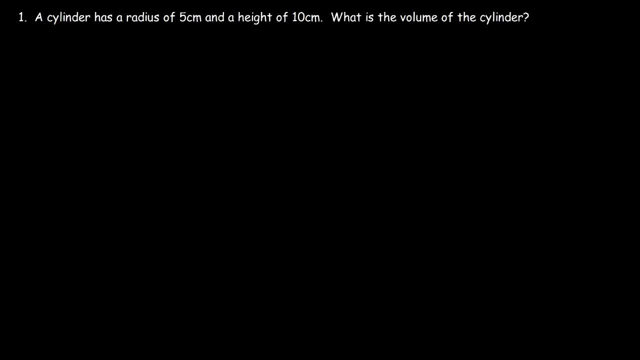 The area that is around the cylinder. So those are the two formulas that you need in order to calculate the volume and the surface area of a cylinder. Now let's work on some word problems. Number one: A cylinder has a radius of 5 centimeters and a height of 10 centimeters. 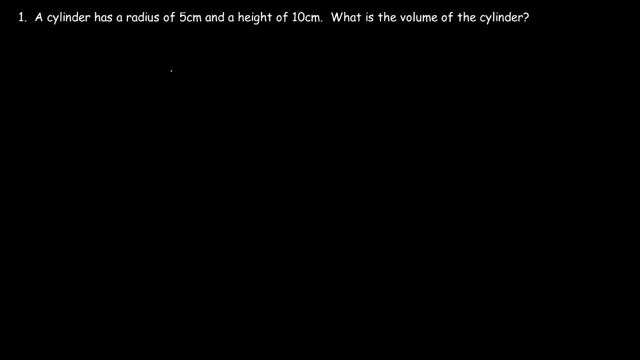 What is the volume of the cylinder? So let's draw a picture. So the radius is 5 centimeters And it has a height, And it has a height of 10 centimeters. So all we need to do is basically plug the info that we have into this formula. 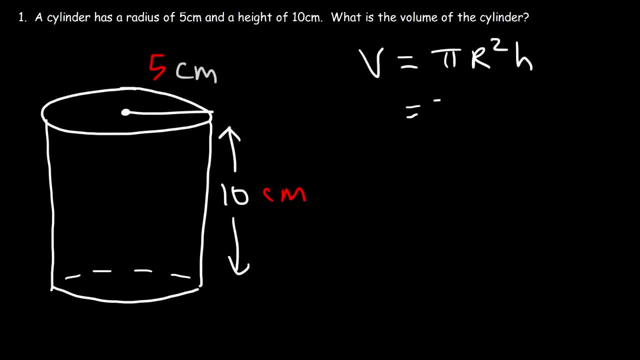 The volume is pi r squared times the height. So it's pi times the radius squared, which is 5 squared times the height of 10.. 5 squared is 25.. And 25 times 10 is 250.. So the volume. 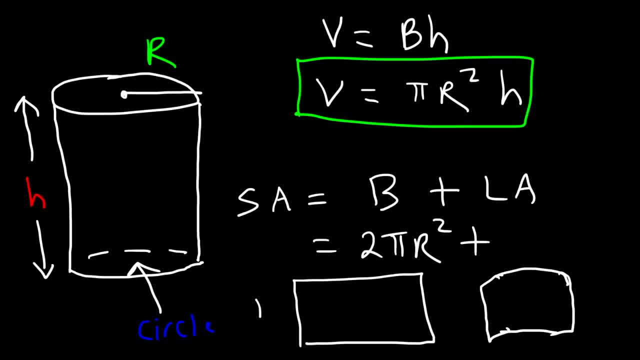 That is the lateral area And we know this is H, And the length. if you turn it into, if you roll it up into a cylinder, that length highlighted in green becomes the circumference of the cylinder. So basically it's the perimeter around the circle. 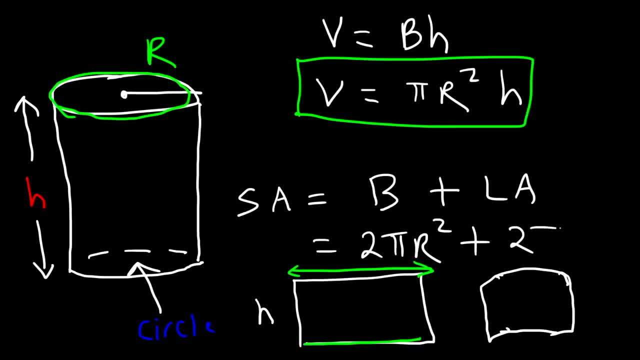 So therefore it's going to be the circumference, 2 pi r, Which represents the length in green times the height. So that is the surface area. It's basically the area of the base, That is, the area of the circle on top and the bottom, plus the lateral area. 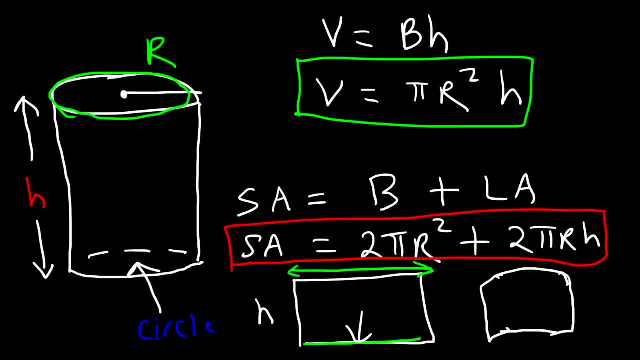 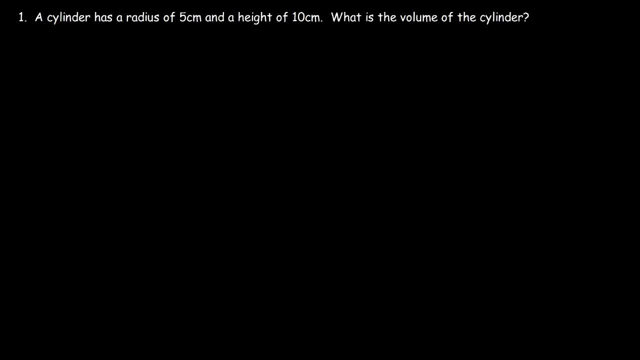 The area that is around the cylinder. So those are the two formulas that you need in order to calculate the volume and the surface area of a cylinder. Now let's work on some word problems. Number one: A cylinder has a radius of 5 centimeters and a height of 10 centimeters. 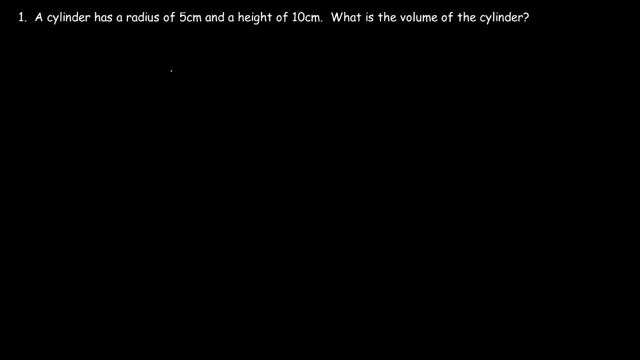 What is the volume of the cylinder? So let's draw a picture. So the radius is 5 centimeters And it has a height, And it has a height of 10 centimeters. So all we need to do is basically plug the info that we have into this formula. 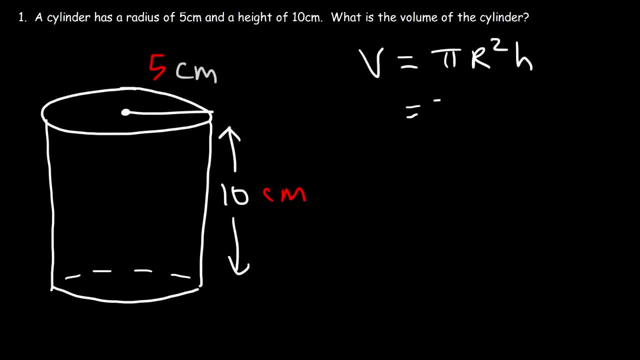 The volume is pi r squared times the height. So it's pi times the radius squared, which is 5 squared times the height of 10.. 5 squared is 25.. And 25 times 10 is 250.. So the volume. 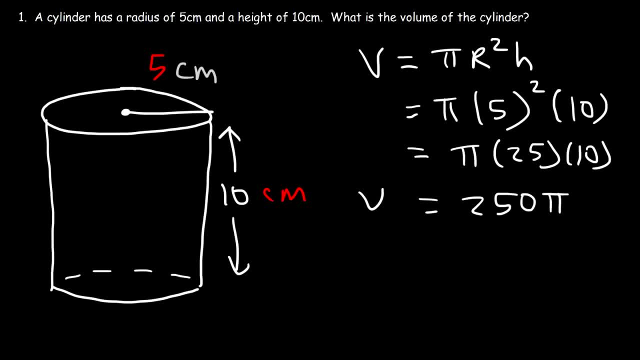 Is 250 pi. So this is the exact answer. You can also write the answer this way: 250 times pi is 785.40.. And the units: cubic centimeters. So you can also write the answer like this, if you want to. 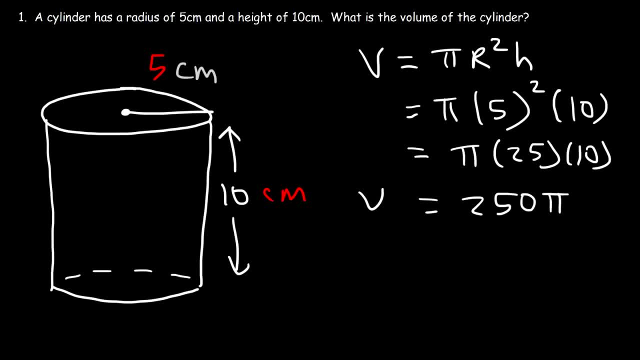 Is 250 pi. So this is the exact answer. You can also write the answer this way: 250 times pi is 785.40.. And the units: cubic centimeters. So you can also write the answer like this, if you want to. 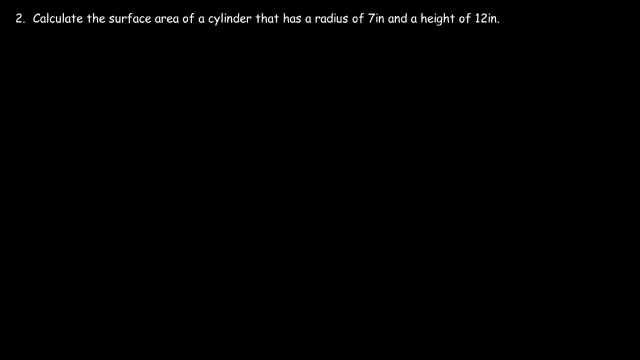 Number two: Calculate the surface area of a cylinder That has a radius of 7 inches And the height of 12 inches. So r is 7 and h is 12.. Now let's write the formula: The surface area is 2 pi r squared. 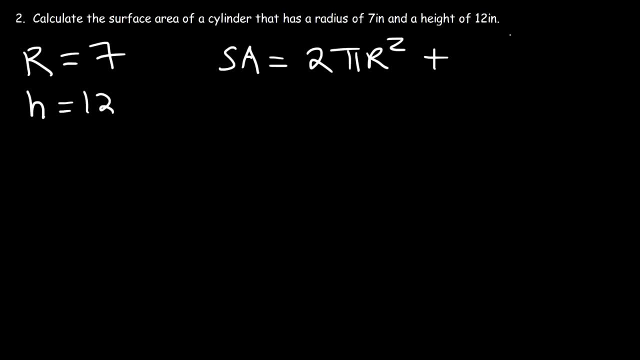 Plus 2 pi r times 5, squared Times 5. Right H? all we need to do is basically plug in everything that we have into that formula. so R is 7 and H is 12. 7 squared is 49 and 7 times 12 that's 84, 2 times. 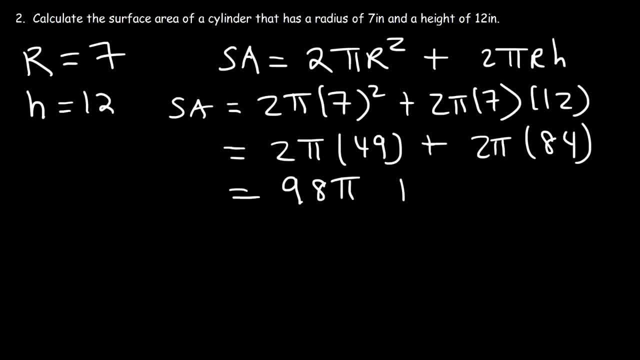 49 is 98 and 2 times 84 is 168. so now what we need to do is add 168 and 98 together. 8 plus 8 is 16, 1 plus 6 is 7. 7 plus 9 is also 16. carry over the 1 and so. 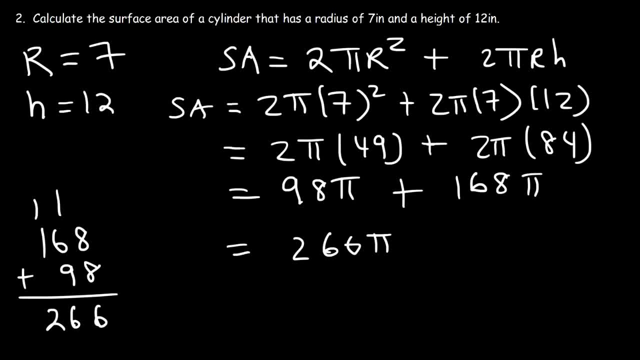 this is going to be 266 PI. so that's the surface area. if you want an exact answer, you, if you want to round it to the nearest hundredth, 266 PI is about. this is using the exact answer, not 3.14. it's 835 point 6, 6, and the units are inches cube. 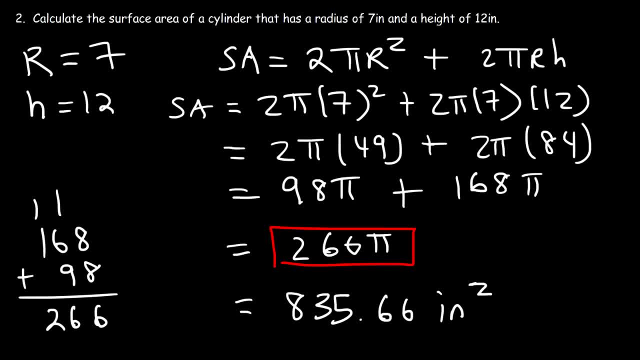 actually inches squared. when you're dealing with volume, it's going to be inches cubed, centimeters cubed. but when dealing with any type of area or surface area, it's going to be inches squared, square feet, square yards, square centimeters, things like that. so this is. 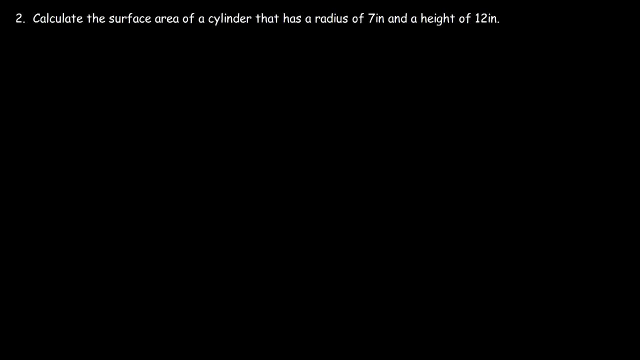 Number two: Calculate the surface area of a cylinder That has a radius of seven inches and a height of 12 inches. So r is 7 and h is 12.. Now let's write the formula: The surface area is 2 pi r squared plus 2 pi r times 5.. 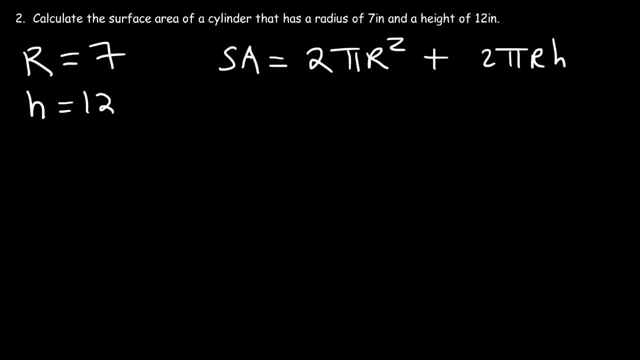 So that is 2 pi r squared, 2 pi r squared, 2 pi r squared. That's right H. all we need to do is basically plug in everything that we have into that formula. so R is 7 and H is 12, 7 squared is 49, and 7 times 12, that's 84, 2 times. 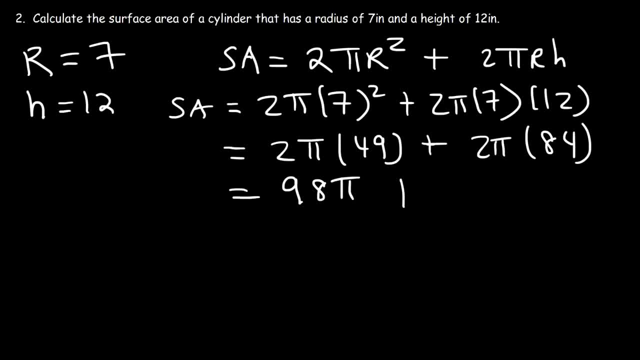 49 is 98 and 2 times 84 is 168. so now what we need to do is add 168 and 98 together. 8 plus 8 is 16, 1 plus 6 is 7. 7 plus 9 is also 16. carry over the 1 and so. 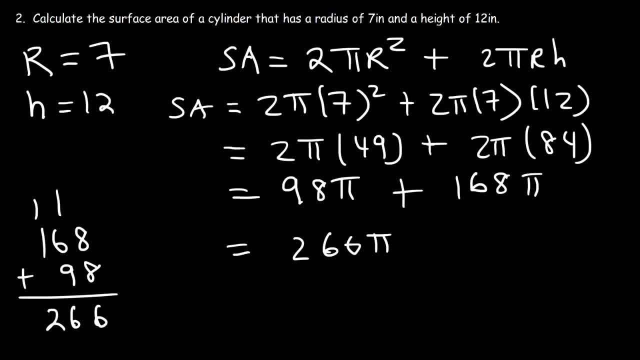 this is going to be 266 PI. so that's the surface area. if you want an exact answer, you, if you want to round it to the nearest hundredth, 266 PI is about. this is using the exact answer, not 3.14, it's 835.66 and the units are inches, cube, actually. 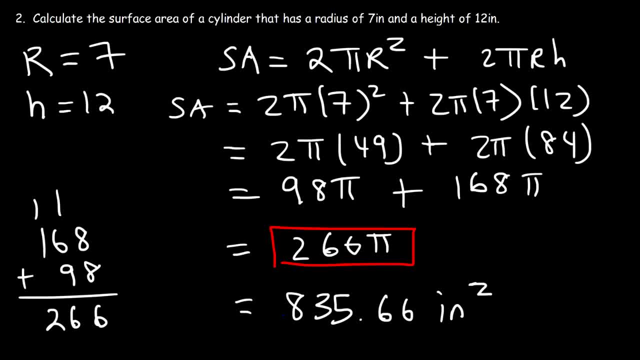 inches squared. when you're dealing with volume, it's going to be inches cubed, centimeters cubed. but when dealing with any type of area or surface area, it's going to be inches squared. square feet, square yards, square centimeters, things like that. so this is 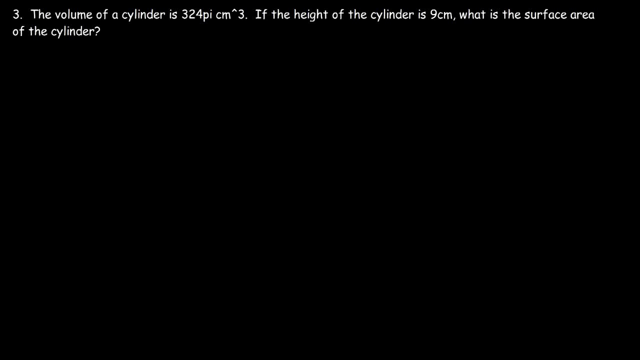 the answer. you can write it in any of these two ways. number three: the volume of a cylinder is 324 PI cubic centimeters. if the height of the cylinder is 9 centimeters, what is the surface area of the cylinder? so take a minute and try this problem. it's best to write down. 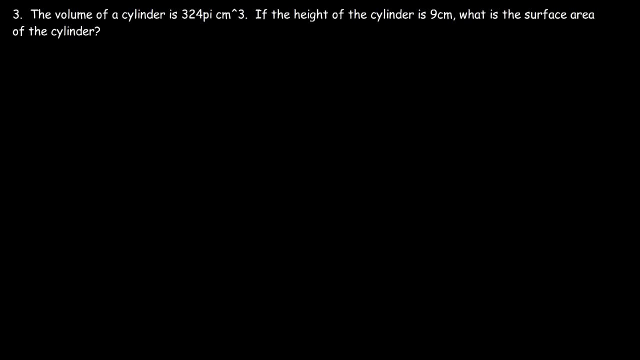 the answer. you can write it in any of these two ways. number three: the volume of this cylinder is three hundred twenty four pi cubic centimeters. if the height of this cylinder is nine centimeters, what is the surface area of the cylinder? so take a minute and try this problem. it's best to write down the 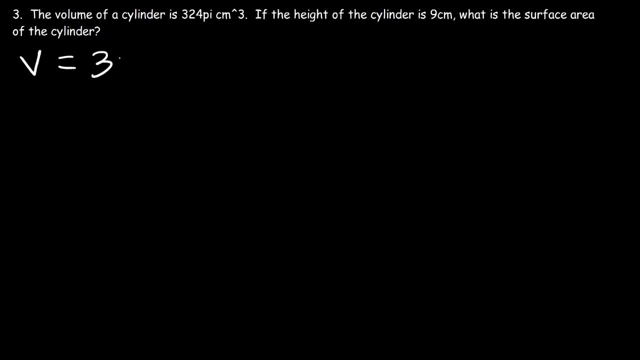 the information that you have. So we have the volume, which is 324 pi, and we have the height, which is 9 centimeters. Our goal is to find a surface area of the cylinder. Now we have the volume equation of the cylinder. it's pi- r squared times. 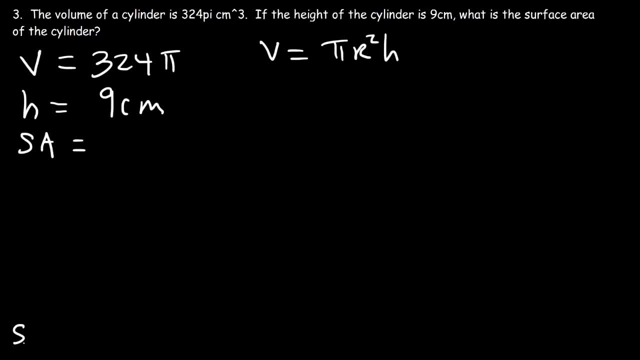 the height and the surface area equation is 2 pi r squared plus 2 pi r times h, So will also missing the radius and needs to find r before we could find a surface area. So let's use this equation to find the value of r first. The volume. 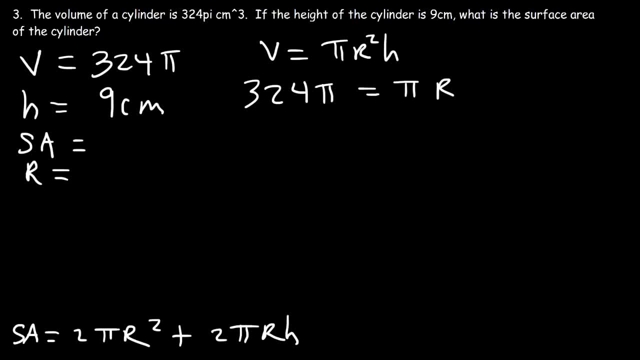 is 324, pi and h is 9.. So the first thing we could do is we can cancel pi. You can divide both sides by pi if you want. Next, let's divide both sides by 9.. 324 divided by 9 is 36.. So 36 is equal to r squared. Now all we need to do is take the square. 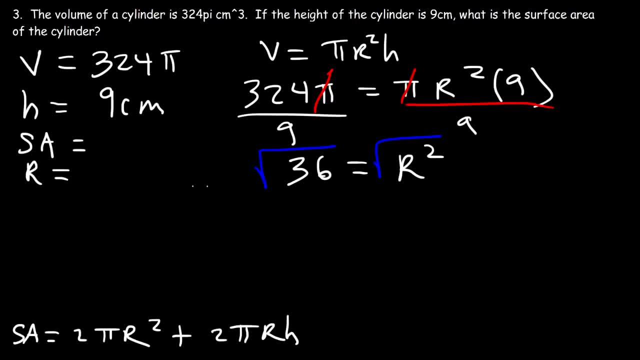 root of both sides. The square root of 36 is 6.. So now that we have the value of r, we can now find the surface area. So the surface area is going to be 2pi times 6 squared, plus 2pi times 6 times a height of 9.. 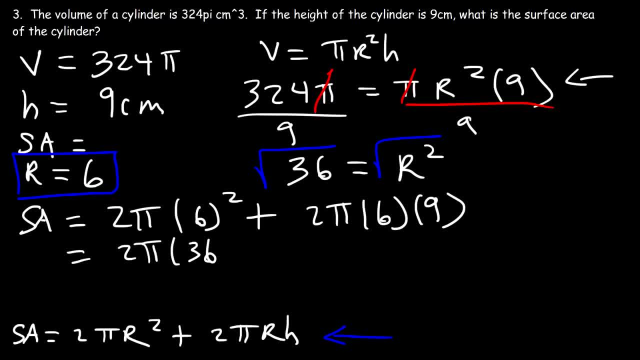 6 squared is 36.. And 6 times 9 is 54.. 2 times 36 is 72.. 2 times 6 is 100.. 2 times 3 is 3.. 2 times 3 is 7.. 2 times 3 is 2.. 2 times 3 is 1.. 2 times 4 is 1.. 2 times 3 is 1.. As we did before, 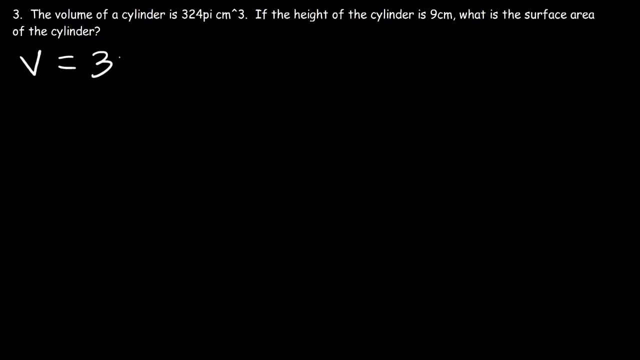 the information that you have. so we have the volume, which is 324 pi, and we have the height, which is 9 centimeters. our goal is to find a surface area of the cylinder. now we have the volume equation of the cylinder. it's pi- R squared times. 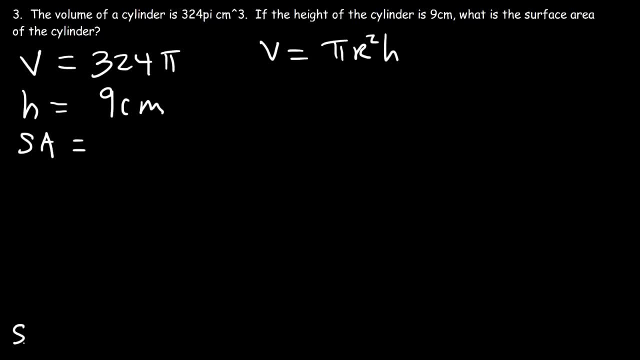 the height and the surface area equation is 2 pi R squared plus 2 pi R times H, so also missing the radius. we need to find R before we could find a surface area. so let's use this equation to find the value of R first. the volume is 324 pi. 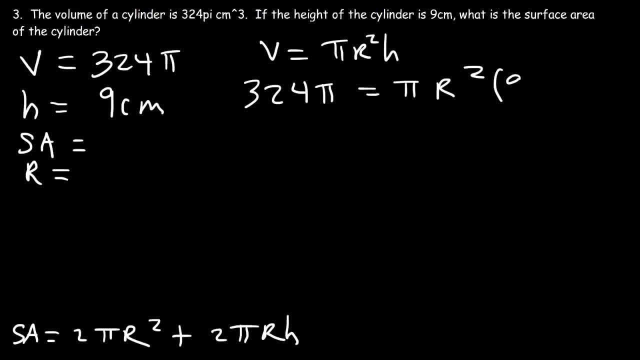 and H is 9. so the first thing we could do is we can cancel Pi. You can divide both sides by pi if you want. Next, let's divide both sides by 9.. 324 divided by 9 is 36.. So 36 is equal to r squared. 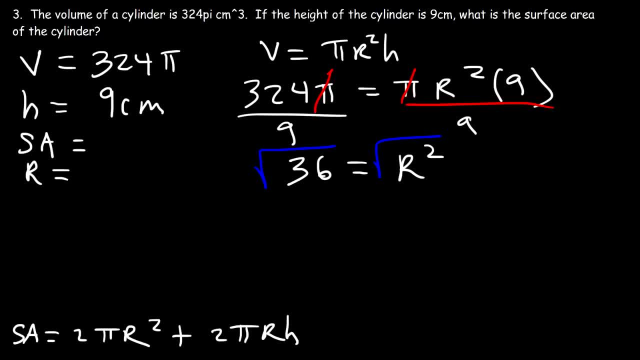 Now all we need to do is take the square root of both sides. The square root of 36 is 6.. So now that we have the value of r, we can now find the surface area. So the surface area is going to be 2 pi times 6 squared, plus 2 pi times 6 times a height of 9.. 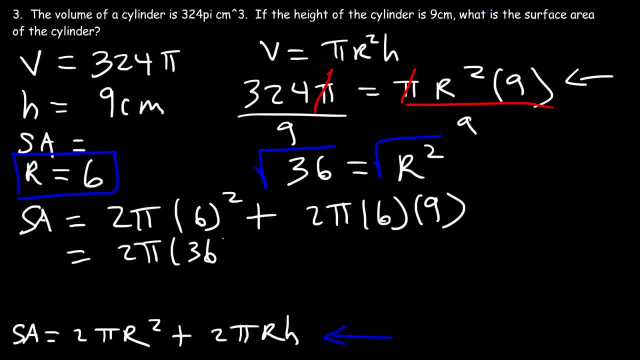 6 squared is 36.. And 6 times 9 is 54.. 2 times 36.. 6 is 72.. 2 times 54 is 108.. 72 plus 108 is 180.. So the answer is 180 pi. 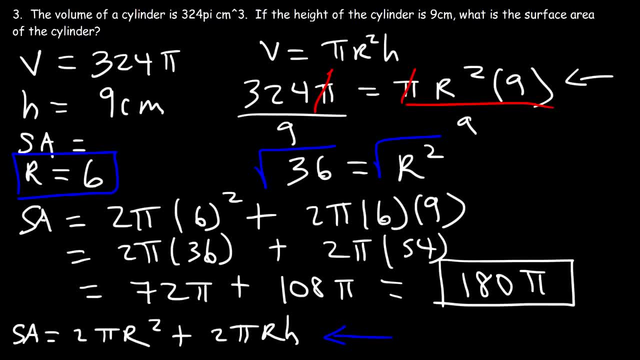 Now, if you want to get the decimal equivalent of that answer, that's going to be 565.49.. And because we're dealing with area- surface area- the units will be square centimeters, And so you can take the area from Products X: prescribe matrix.